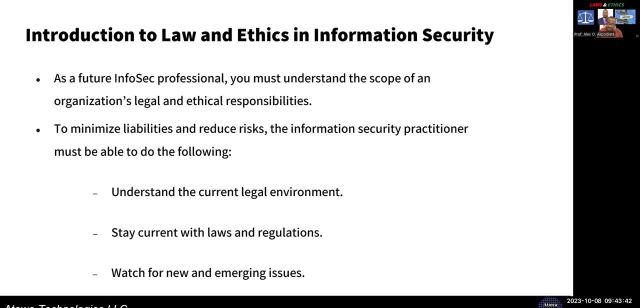 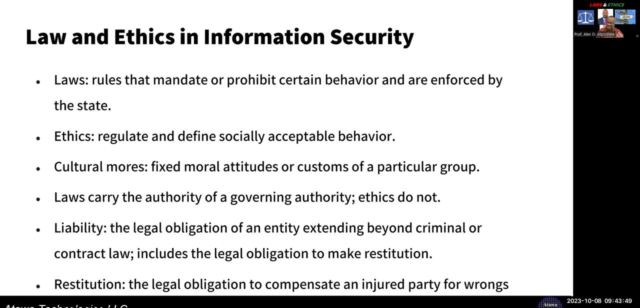 by trying to, of course, look at your current legal environment, And you should stay current with the laws and watch for new and emerging issues, right. So for about 16 years I spent career as an attorney, practicing both in US federal and state court and some international 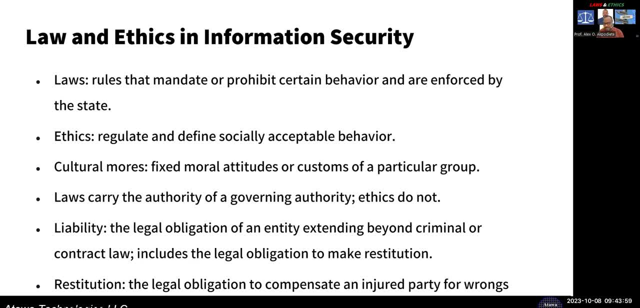 cases And I'm going to go across the border and then try to explain to people what this means for them and what this doesn't mean for them. I used to teach specifically from, I think, Korea, US and other places on issues of what we call the legal aspects of doing business in the US. 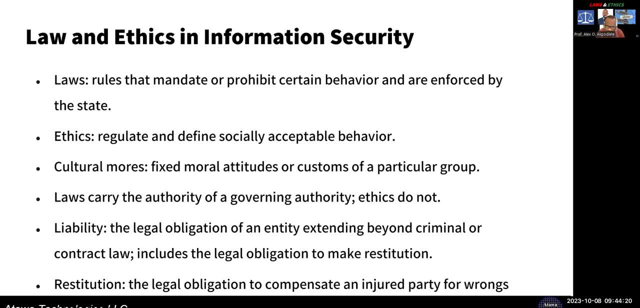 And then my first foray into formal academia was as a professor of business law and ethics, So this is actually talking about. well, 22 years later, to really do this video. So laws basically are enforced by the state and it's compulsory- or you say the word, mandatory. 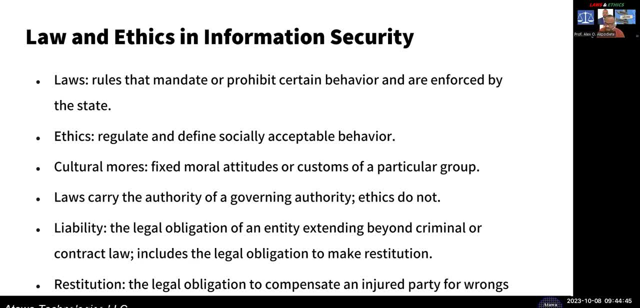 Usually in the democratic system, you have three branches of government right- The executive, the legislative and the judiciary- And you'll be told that the judiciary is the one that makes law and that the executive enforces it. But when the so, the legislative branch makes the law and then the executive is supposed to enforce it. Well, 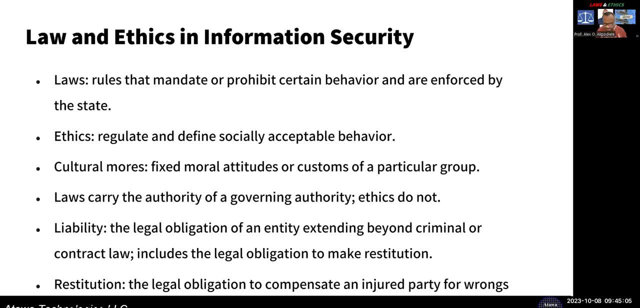 however, when the judiciary make, even interpret, an act or a portion of the constitution, they're also making the law. But the process is: your legislator will draft the bill and then the bill gets voted on, goes through reading before it comes before the House of Reps or the House of 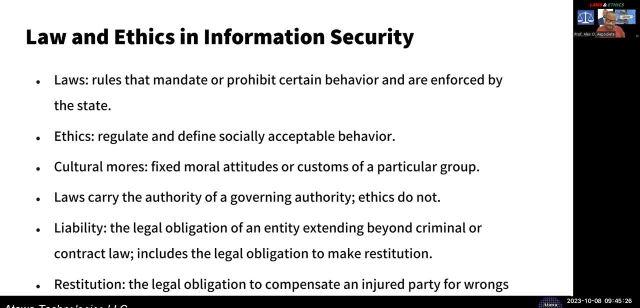 Senate or House of Lords or House of Commons, whatever you have in your own area, or the House of Assembly. So the House of Lords, whatever you have in your own area, or the House of Assembly, and then they vote and it now goes to the governor or the president to be signed into law Once it's 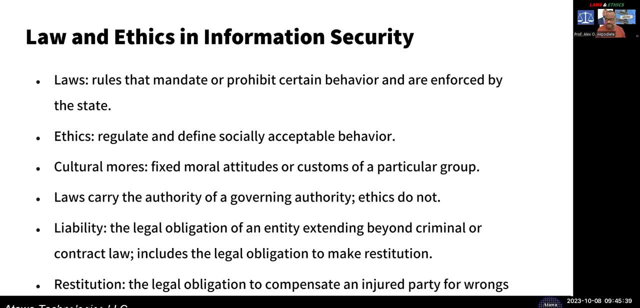 signed. it becomes an act If the president, for example, does not agree with it and he can now veto the bill. But many societies or many countries have a rule that says two-thirds majority of the legislative branch can override the veto of the president and it still becomes law right. So if 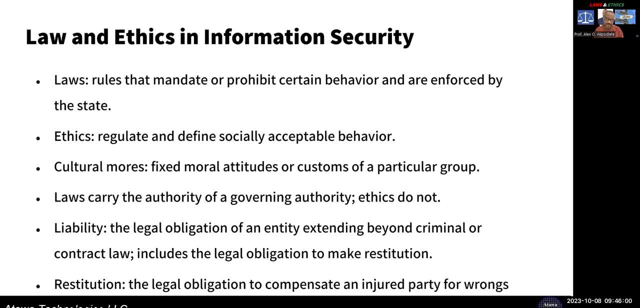 you're reading an act, you will see on the bottom whether it was signed by the president or not. right Ethics, on the other hand, are basically what we call things to regulate your behavior socially. The word cultural morals be like moral attitudes. So for law, whether it be administrative, 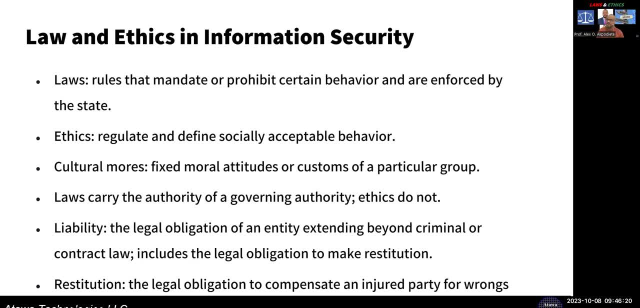 law, civil law, criminal law- there are consequences to violating them right. In the case of a civil law, which would be either corporate law for business or what's called tort, like negligence- hitting somebody with your car- or assault- Because even assault could be both criminal and civil right- You get a fine. 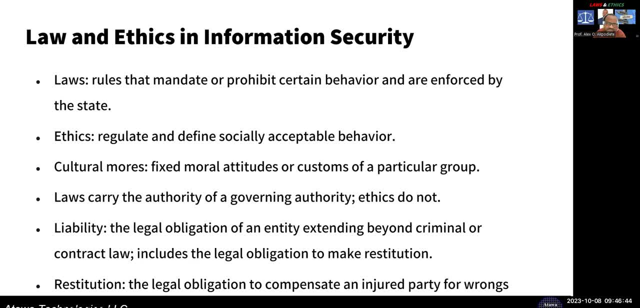 you get a monetary judgment, which is how most of us made money as a lawyer- And then the criminal one. you're going to go to jail. it's less than a year in most places. it's called a misdemeanor or felony if it's more than a year, right. So sometimes you have restitution. 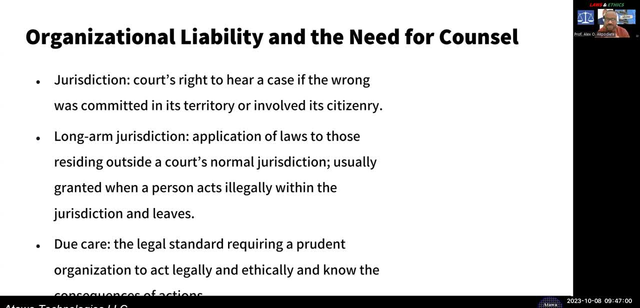 you have to pay back money for that. So the word jurisdiction means the right or the authority of a court to hear your case, And there are two types of jurisdiction really: personal jurisdiction or long-arm jurisdiction. I know you don't have one because subject matter jurisdiction, but on here. 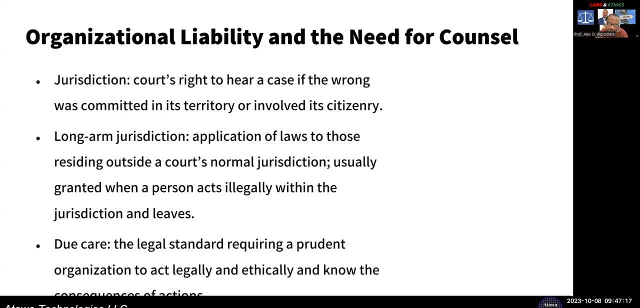 when it talks about long-arm jurisdiction, see, it's for laws that apply to those who are not even in the court's jurisdiction right, But because maybe you did something within that jurisdiction or your jurisdiction, you have to pay back money for that. So the word jurisdiction means 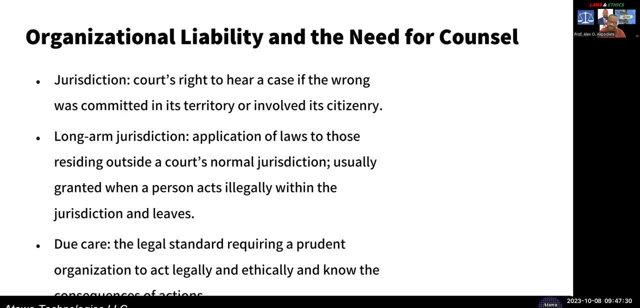 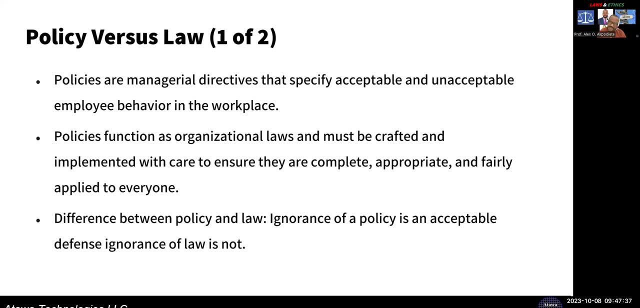 you left or you entered a contract and you agreed right. So you have issues about also due care, due diligence in law. Now they want you to know the distinction between policies and laws. It's kind of like unique, because usually you've heard the expression that says ignorance of the. 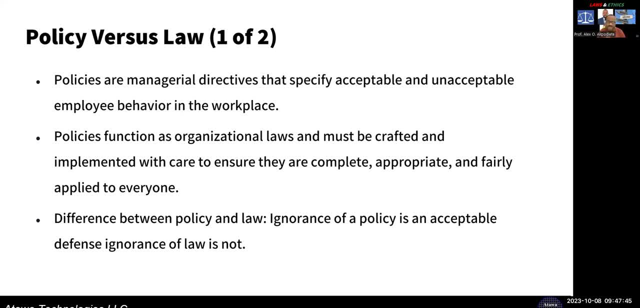 law is not an excuse, but it says ignorance of policies could be an excuse, right? So if you're looking at the hierarchy of what organizations deal with in terms of rules, or you have your- you know your- policies on top. that's normally from a top. 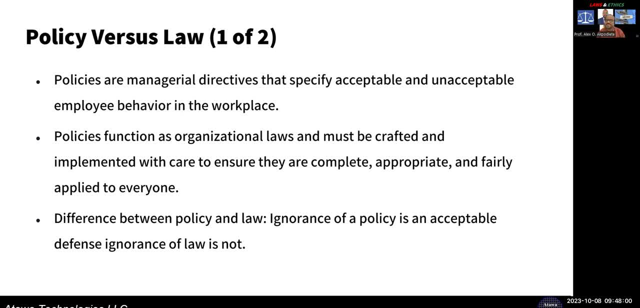 management, or you have strategy policies and, of course, way down to like guidelines, right? So you're just telling that policies here are from the management and they will be considered the laws of your organization. like acceptable use policy technology, what you can do on the internet. 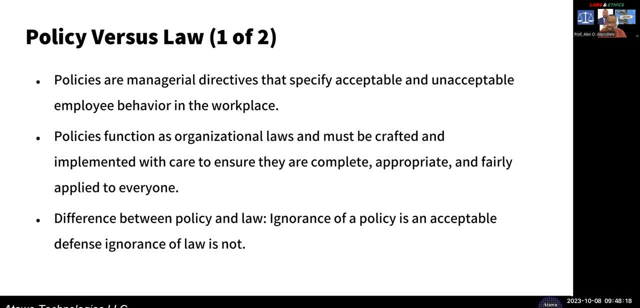 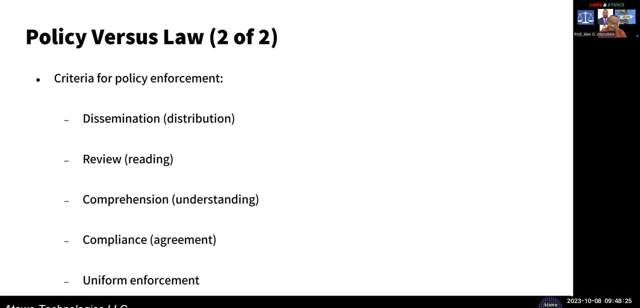 and what you cannot do on that internet using the company's network. right, All right. So for policy to be enforceable, it needs to be disseminated, meaning everybody needs to be able to have access to it. right Reading of it, understand it. 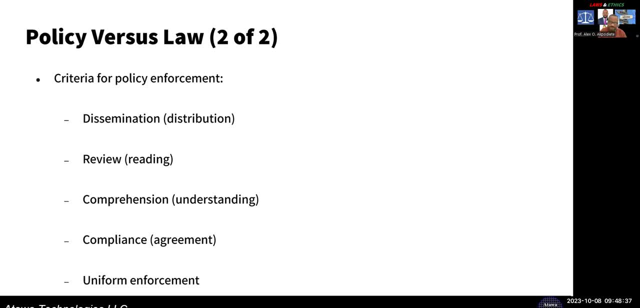 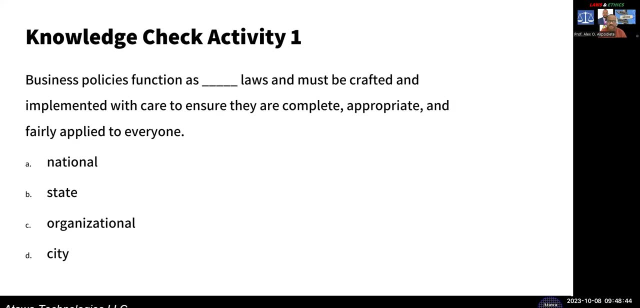 agreement to comply by and, of course, uniform enforcement. these are some attributes of a policy that's required for it to be enforceable. so see this little slide: the knowledge check. so business policy functions as DASH law and must be crafted and prepared with care to ensure they are complete. 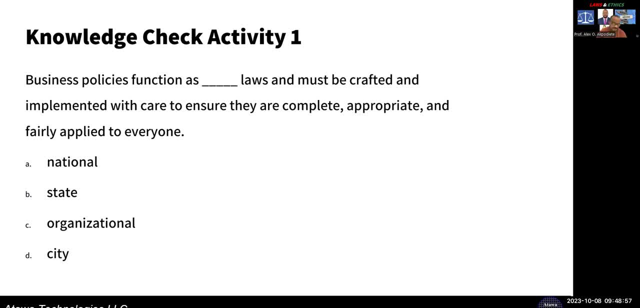 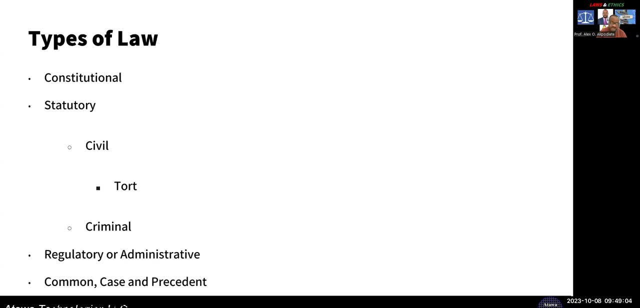 appropriate and fairly applied to everyone, right? So if you're talking about business policies, functions as right, it would be organization right? Alright? so, as I said, there are different types of laws. you got the regulation, so the only thing I didn't touch about was the 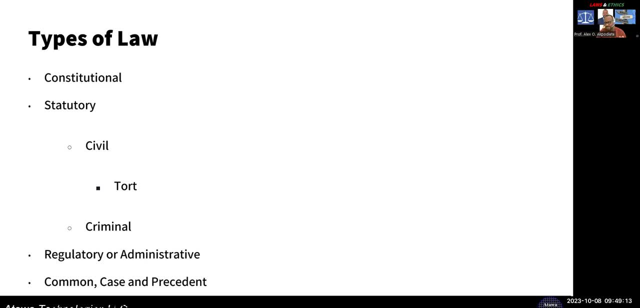 constitution and common law. common law would be for, like former British colonies, like you hear the word common law wife, like just by virtue of living together after so many years you become wives or something it's not really like codified, like written down somewhere, like it says you have to go get. 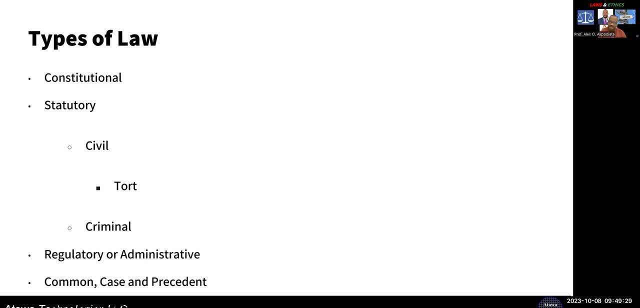 a court certificate to get married, but you might have, maybe have court cases that interpret the living together to mean that you are now legally married after so many years, or in case of property too. if you are squatting on a property after so many years in some jurisdiction you become the. 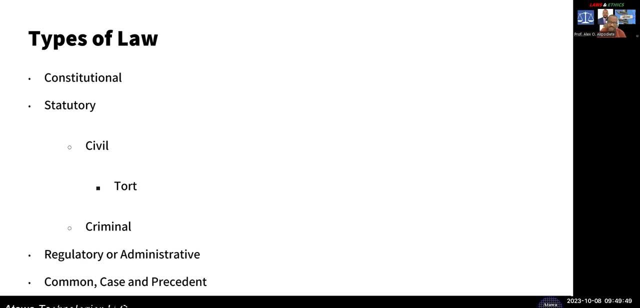 owner of the property. Now, the constitution is considered the supreme law of the land. every other law falls down, falls below it. So you keep that in mind. if you ever hear somebody ask you what is the supreme law of the land, it tends to be constitution, Any place. 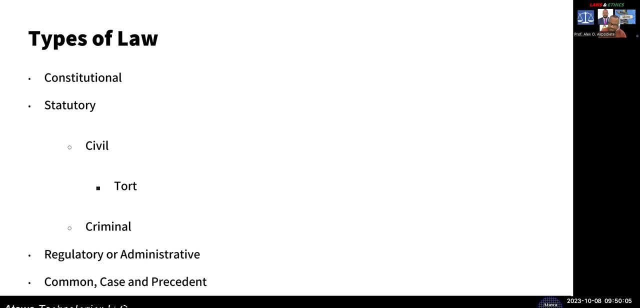 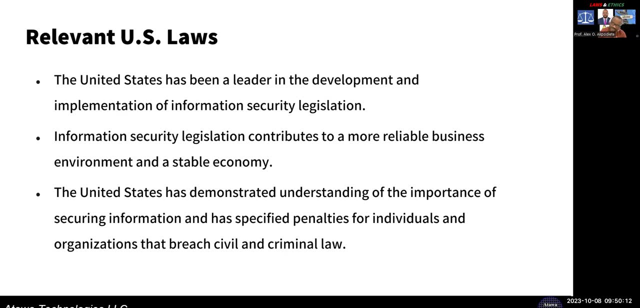 that has constitution right. even with democratic regime or military regime or authoritarian regime, they still have a constitution right. So this is the portion I warned you ahead of time might be very American centric, because if you're watching this from another part of the world, just try and 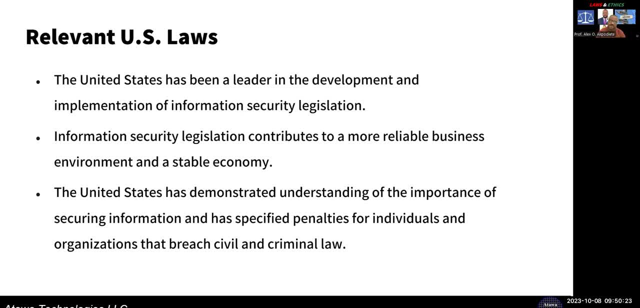 see, is there something comparable in your country? right, So, but the whole idea is because the US has been part of a leader in the development of information security legislation. we have to look at some of their laws as an example. right, Of course, now with the 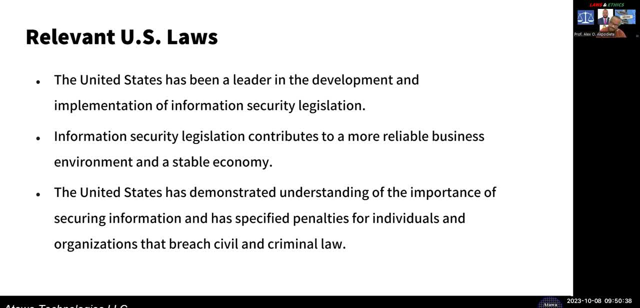 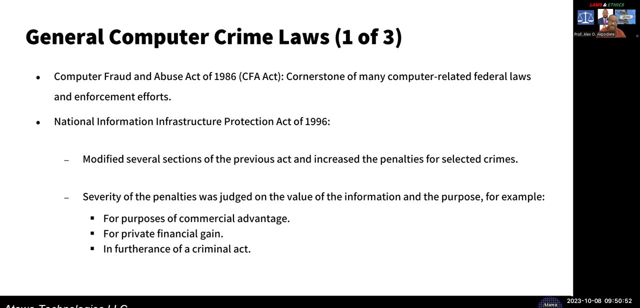 United Nations and other international bodies, they're also having laws that affect information security right. So the reason why the US passes laws: because they want to encourage business in information security perspective. So the first thing here is that computer fraud and abuse act of 1986. 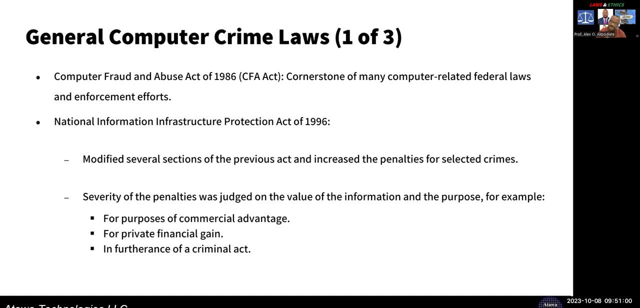 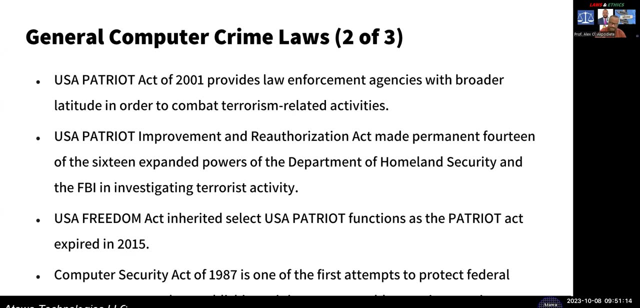 uh, this is you call it the uh. like it paved the way for many computer related federal and federal enforcement laws. You have what's also called the National Infrastructure Protection Act in the US, and then you have the US Patriot Act that grew out of the whole 9-11.. 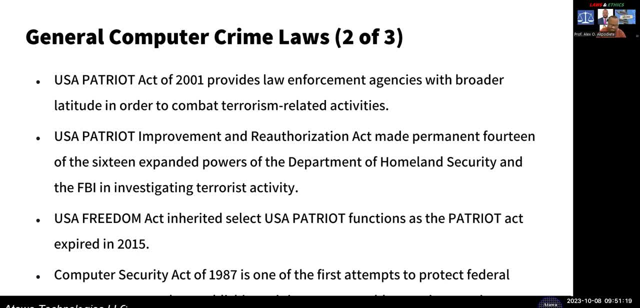 The whole idea here with 9-11 is that you kind of like made permanent 14 of the 16 previously expanded powers of the Department of Homeland Security and FBI investigating like terrorist activity. and they also have the USA Freedom Act and then the Computer Security Act of. 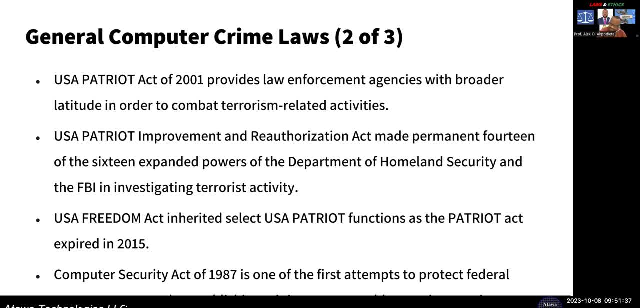 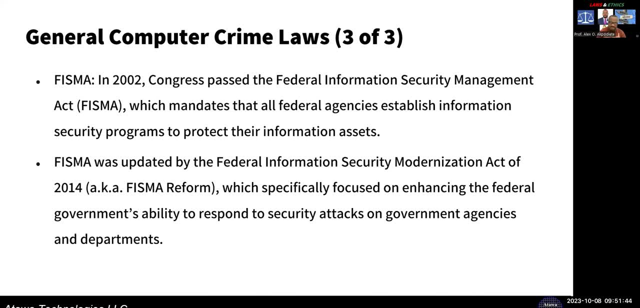 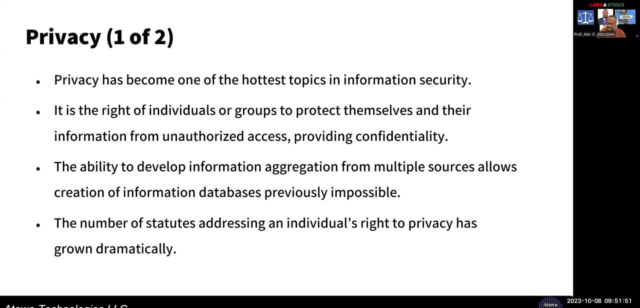 1987 was like the first attempt by the US to look into IT. so you've got FISMA when you have. I hear FISMA mostly has to do with federal agencies. okay, and then, um, let's talk about privacy. So many. 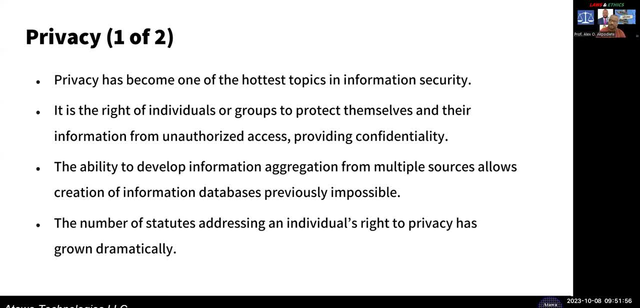 countries have their own laws of privacy. uh, if you're in the European Union area- you heard about the GDPR Fan California, you have a California Privacy Act. but the whole idea is this is a very hot topic in cyber security. Quite a lot of my lawyer colleagues. they. 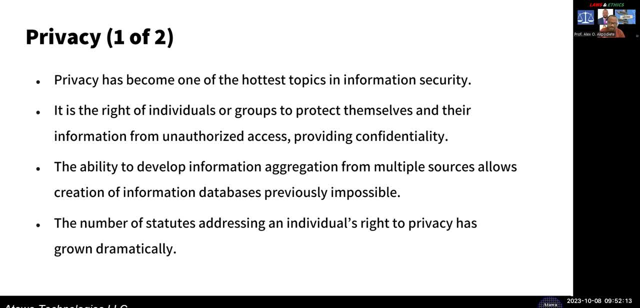 will leave the practice of law and become like data protection officers or get more into a privacy Right. so private World Progressive and Public Trade Authority has about the right to be forgotten. So the whole idea is that every individual or group has the right to be forgotten. So that is about the terms that we го io designate for事情 s. 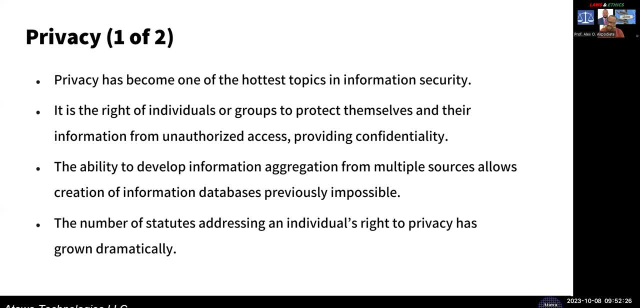 to protect themselves and their information from unauthorized access. in other words- remember the cia tried in cyber security- they want to have a confidentiality right. so there's so many laws now that sometimes it's difficult to keep abreast of them dealing with privacy. so, because there's so, 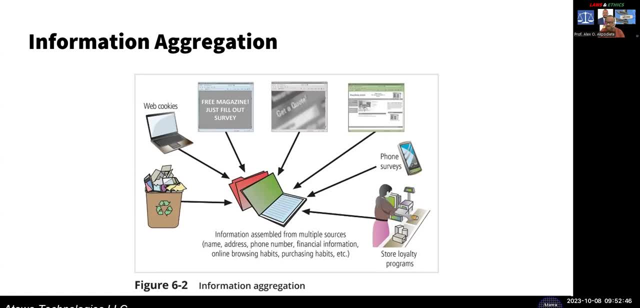 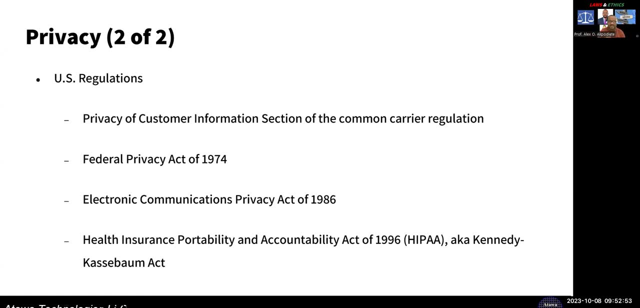 much information coming from everywhere, we need to be concerned, really, about their privacy. so i could have titled this thing laws, privacy and ethics. but you know, because privacy legislation will come under law, that's okay, right? so us regulation, like the privacy of customer information, the federal privacy acts, electronic communication act, and then the hipaa, which is also called the 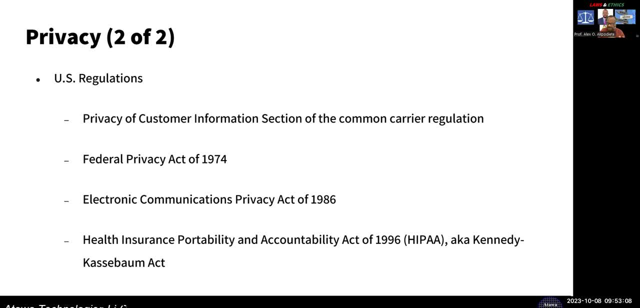 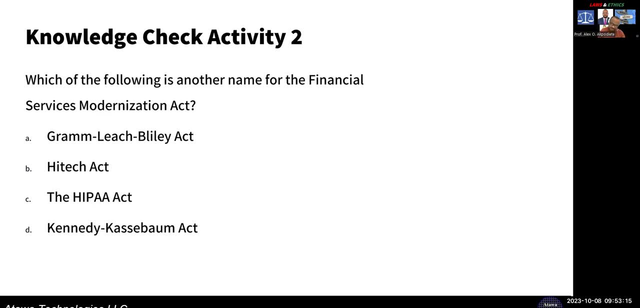 kennedy carlson bomb act has to do with the healthcare industry. it's a very big law in the us protecting healthcare information. so, uh, again, the us centric question, which are the following, is another name for financial service: uh, modernization act. that would be our uh, graham. 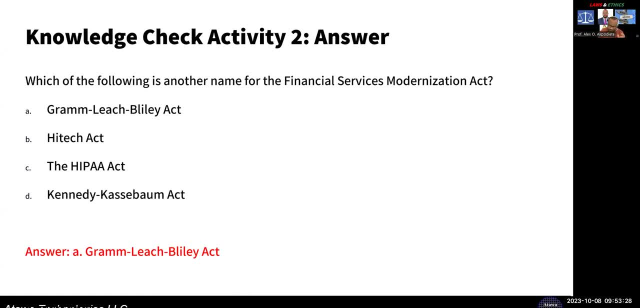 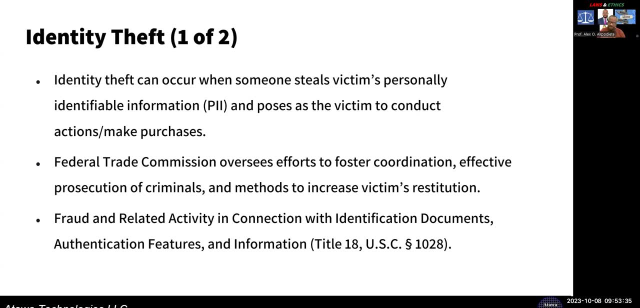 graham leach, uh bailey, act for for us, uh, students. okay, let's talk about identity theft. i have been a victim of identity theft. i was overseas on a contract. when i came back to file my tax return i was like, hey, you already filed your tax return. in fact, we gave you eight thousand dollars. 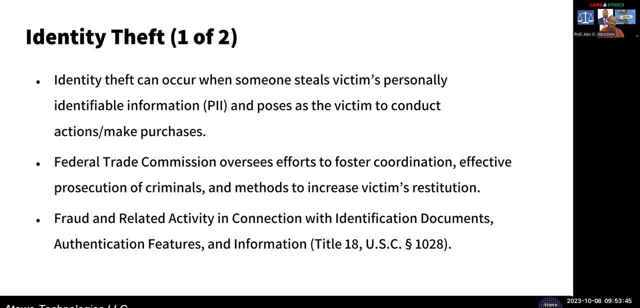 somebody had like solely my information and pretended to be me. so it's, it's very rampant and i remember going to the police and they're like, oh, this happens a lot and the way it happened was considered the the uh mainstay of uh identity fraud in the us right. 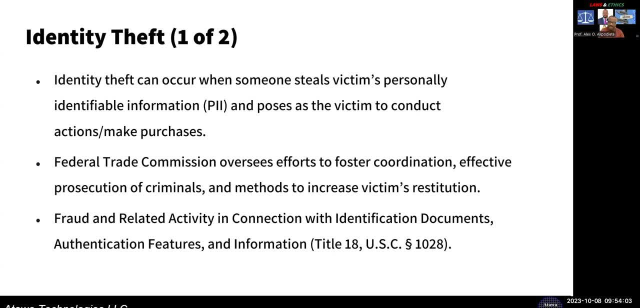 so somebody steals your personal identifier information- pii, maybe a national id number- and then uh poses issue. so the usa ftc has some effort. so what to do? and then the there's another law there. so usually in the us you just report and then you don't use the. 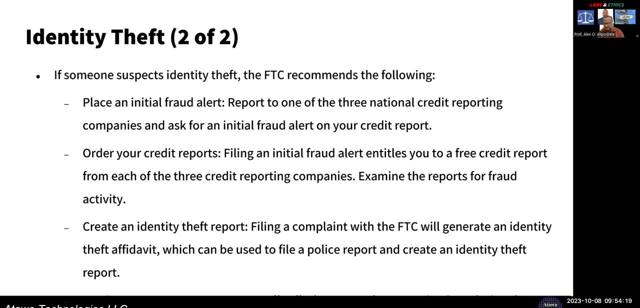 law. you just report and then and it just basically fraudes the equipment to cover it. so one can sue then and you can show, you can call it or not for it, and if you don't know what you would count in here And then the check- in my case the check. they'll be like: okay, we know, it wasn't you. 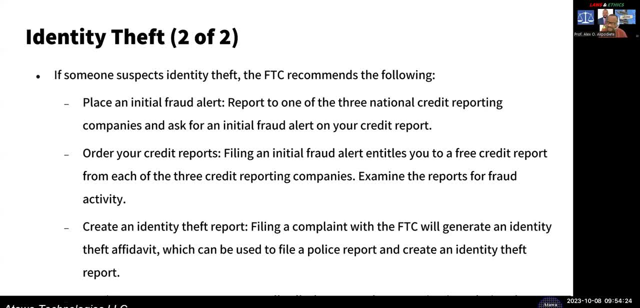 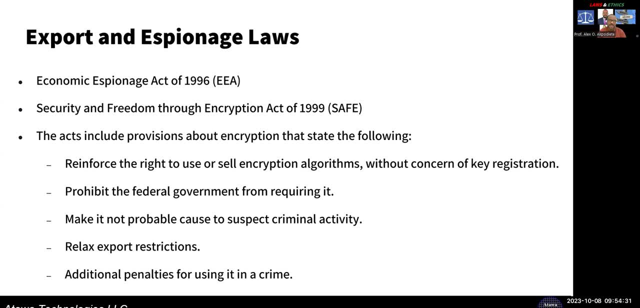 But that means if you want to do certain things, you need to notify the US government or get a special code right. This is what you do if you suspect that you've been a victim of identity theft. So now this is your economic espionage act law. 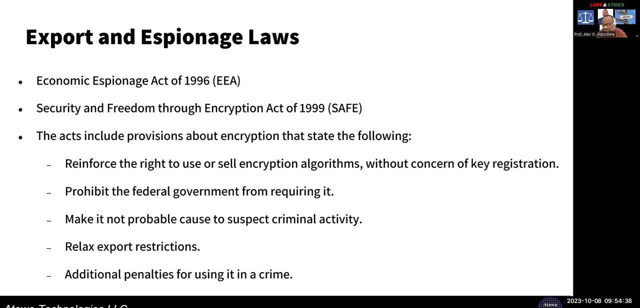 You'll hear people saying that one particular country in Asia is very good at spying on systems. They will plant malware and they will stay there and they'll steal your information. So you have acts to cover that. It's the purpose of commercial espionage. 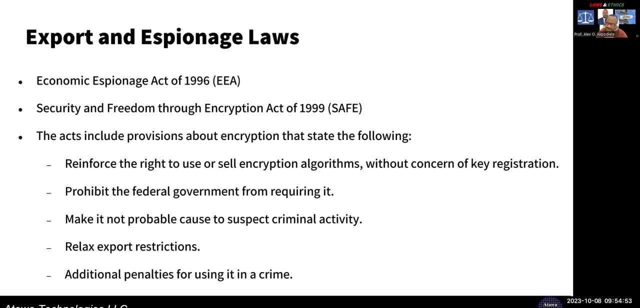 And then you've got the encryption act. There's something that's not covered here, but there's people that do like foreign consulting. There's something called ITAR- International Transport of Arms Regulation. You'll be aware of it. It's going to be teaching like cybersecurity. 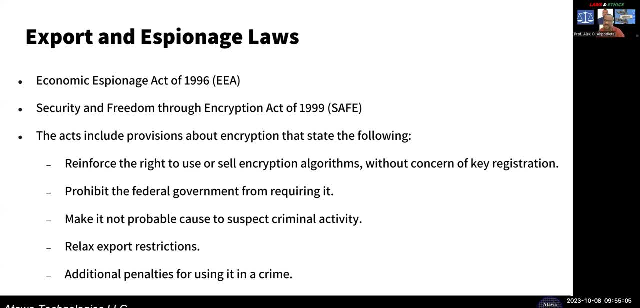 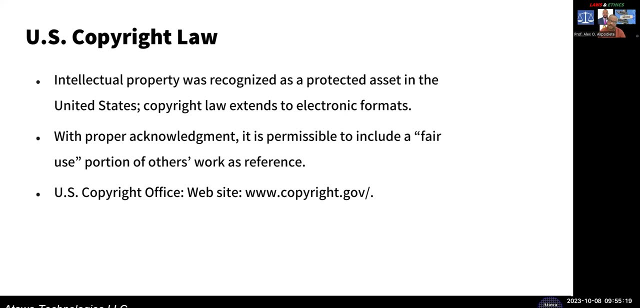 You'll be like: why cybersecurity governed by arms regulation? Just know that it is governed. You need to be careful what you do when you're teaching, like hacking or ethical hacking in different parts of the world. right, All right, so let's use intellectual property IP, not for internet protocol IP as well as intellectual property. 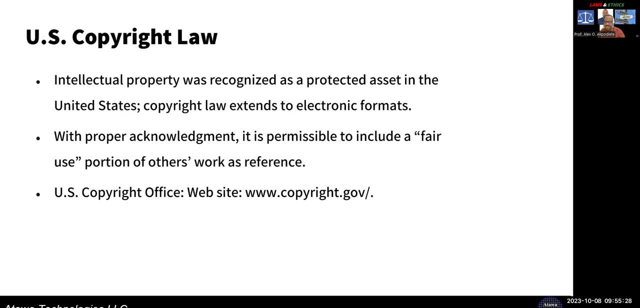 There are really four types. You've got your trade secrets for your business. You've got your copyright for your written work. You've got your trademark. I might miss this one. I mean patent for invention. Those are the four general areas you should be aware of for intellectual property right. 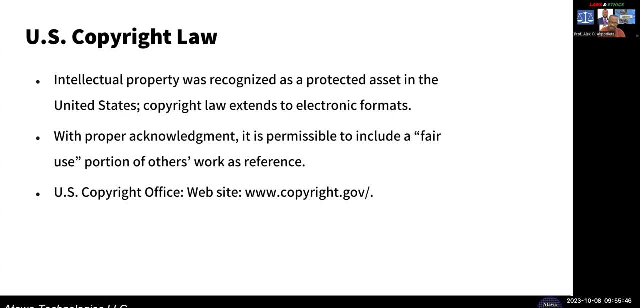 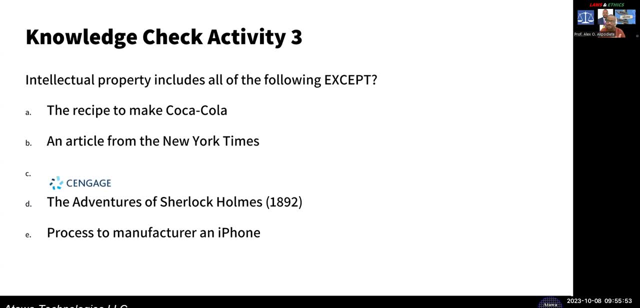 It's protected under US law, So you can, But there's Exclusions for fair use, right? That's a website. So what happens with copyright is sometimes you have to register your copyright in more than one jurisdiction to make sure you don't become a victim. 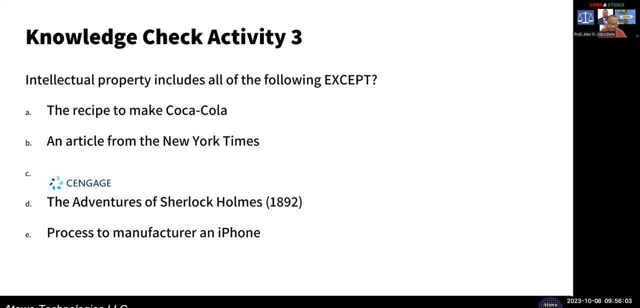 And there are international copyright regulations that you should probably be aware of, But that's another class here. So this is a question to. intellectual property includes all of the following except the recipe to make cook, an article from the New York Times. This is Cengage. 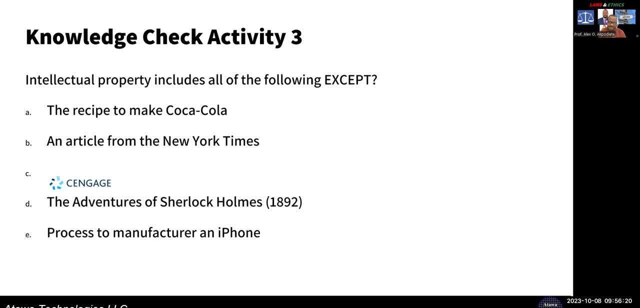 Logo for a company that we use their books, Also the adventures of Sherlock Holmes, and then the process to manufacture an iPhone. You will be surprised about the answer. The answer here is the adventures of Sherlock Holmes, because copyright has a fixed period of time. 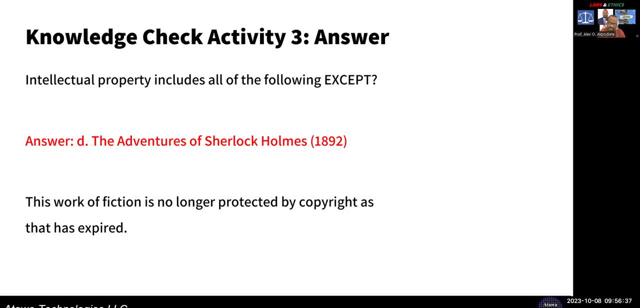 In this case the work of fiction is no longer protected by copyright because it has expired. Send you some of the patent to you. have a reasonable amount of time depending on your country- how many years you can enjoy The fruits of your invention. 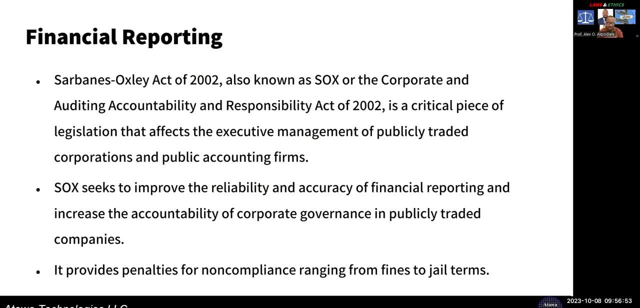 All right. so, Sabine Oxley, you might not be aware of the Enron, but just know that this was came out of issues about concerns about what auditing firms were doing publicly accounting- public accounting firms. I happen to have worked for Pricewaterhouse, but this didn't cover Pricewaterhouse. 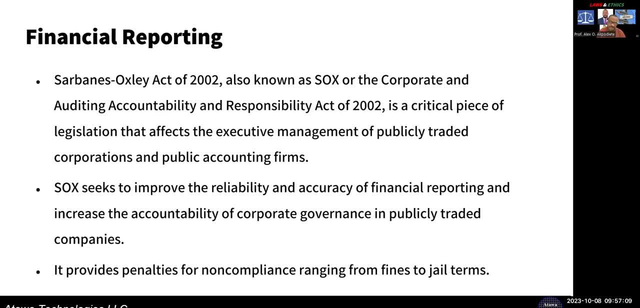 It's for another accounting firm, right. So the whole idea here is that. so you hear Sabine Oxley is called SOX right? So how do we make sure that we're doing the right thing? So you hear Sabine Oxley is called SOX right. 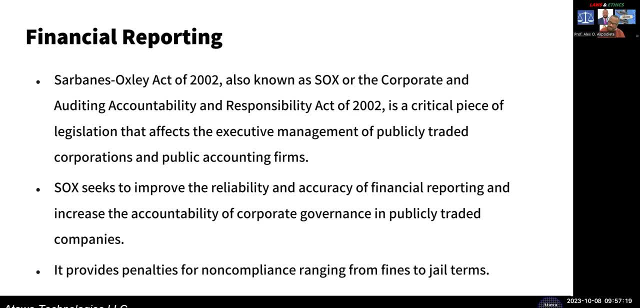 So how do we make sure that we're doing the right thing? So how do we make sure that we're doing the right thing? So how do we make sure that accounting information is provided by a publicly traded company is accurate, so that there's penalties for noncompliance? you can pay money or you can go to jail. used to be for accounting firms to just do and don't have any liability, or the CEO just sign like a public disclosure tax. 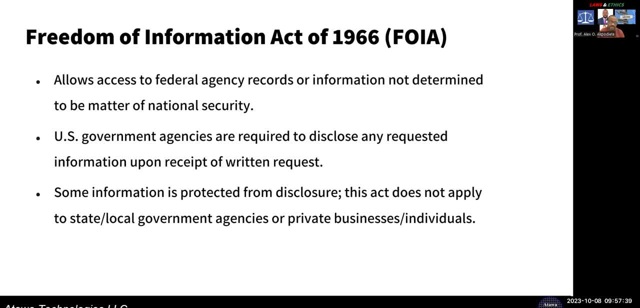 Now you can be personally liable for signing those documents. So Freedom of Information Act, which you hear the word, we, as an attorney, we call it FOIA- allows us to have access to. So Freedom of Information Act, which you hear the word, we, as an attorney, we call it FOIA- allows us to have access to. 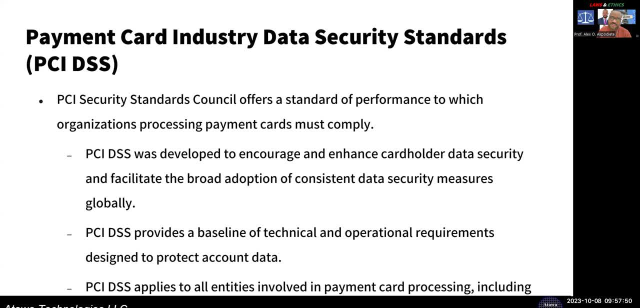 So Freedom of Information Act, which you hear the word, we call it FOIA- allows us to have access to. So this you're going to encounter a lot in your cybersecurity or privacy or InfoSec career, which is the PCIDSS, the payment card industry data security standard. 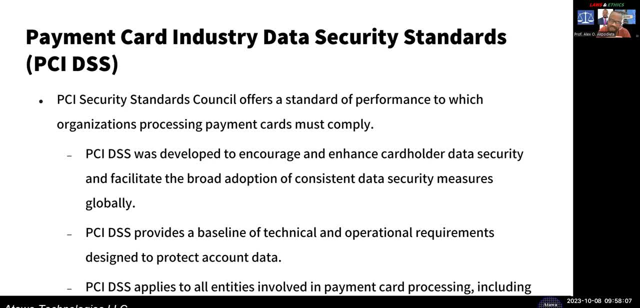 It's actually not a law. it's more like a voluntary compliance with some kind of guideline, right? So the whole idea is to encourage anybody or any entity that processes debit card or credit card to adopt certain security features, right? so you call it. 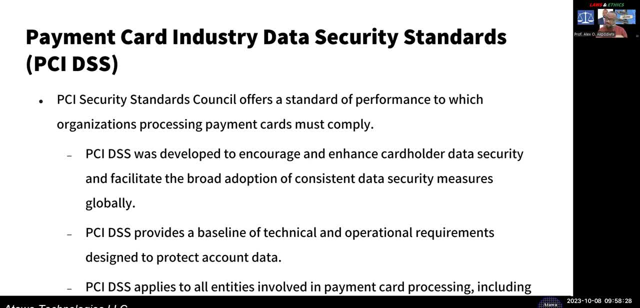 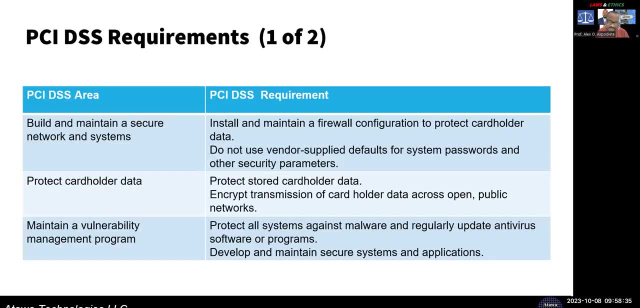 consistent data security measures. so there's a kind of- uh, what's called technical baseline and operational requirements. so anybody that processes a credit card must abide by this. so this is a chat about some of the areas and the requirement right: protect your cardholder data and encrypt. 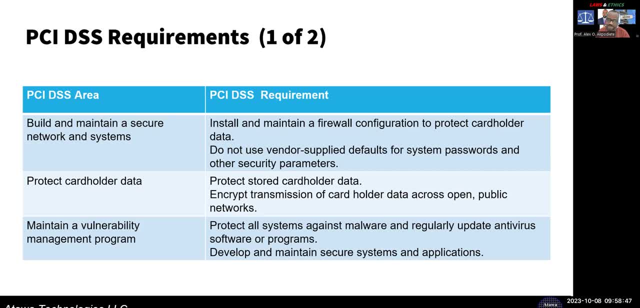 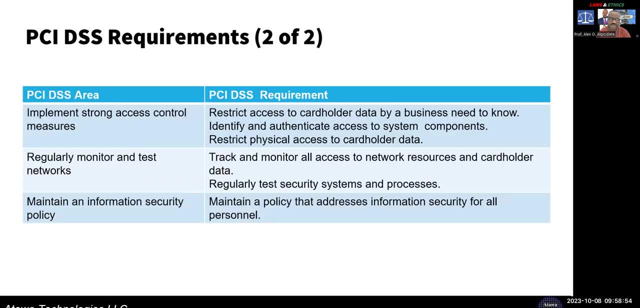 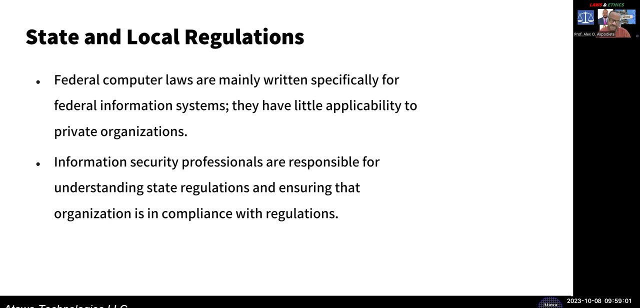 transmission of the card across open public network. so the maintain your vulnerability management program, right. have an infosec policies, all right. so state and local regulations- I can also add international here- so you have federal laws and also you have to be aware of your state laws, right. so if you're practicing as a cyber security analyst, infosec professional, you have. 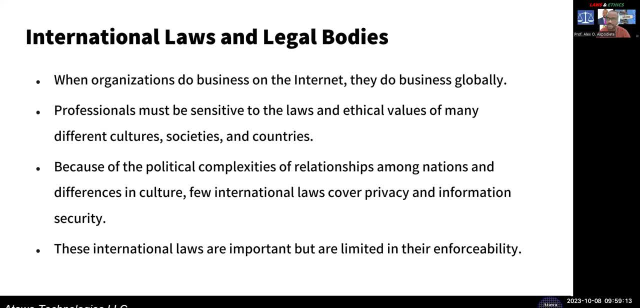 the responsibility to understand the state regulations and make sure that you are in compliance with it. um, but the issue? so now, for example, now, cyber crime. there really is no international agreement on cyber. there's something called the Budapest Convention, but not all countries have signed to it, right? but imagine this: I'm so, I'm sitting at this, this video, I'm making this video today from 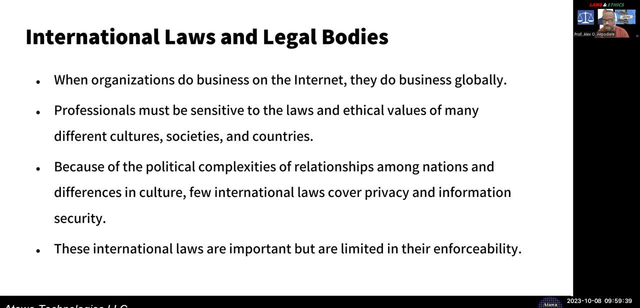 Dubai. so let's say, I use my crime, my computer, to commit a crime on the internet against somebody in America. so, uh, which law is going to apply to me? the law of the United Arab Emirates or the law of the United States of America? so you can see there are issues, right, because there may be complexities of countries. 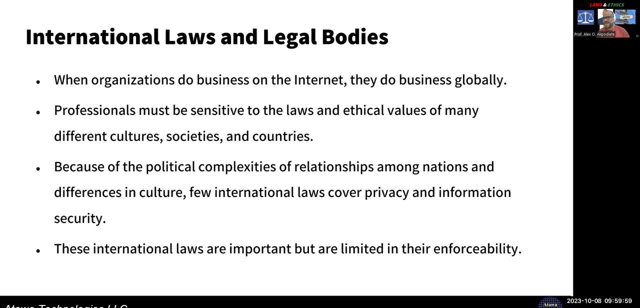 just know that there are. I, for example, if I'm carrying a like jammers, for example, are illegal, right for jamming signals. but maybe some countries might just allow you to go by. some countries they see, or they see hacking tools with you. you're going to go to jail, so just be careful. right to 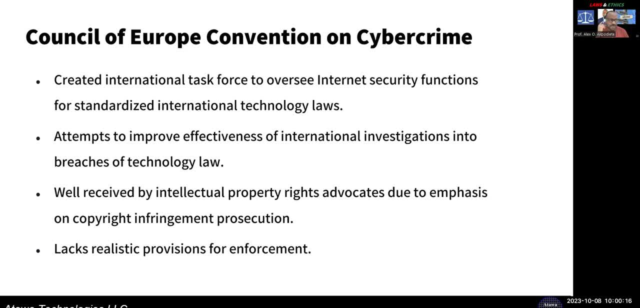 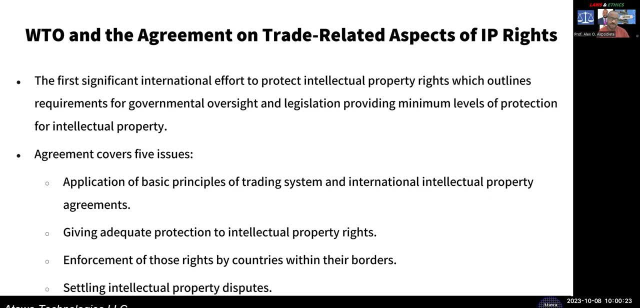 know about international law, right? so you have a Council of European Convention on cyber crime. they made some attempt, but the question is: how can you enforce the law? and then the world trade organization also has, uh, some aspects related to, uh, intellectual property, and which means also related to tech, right? so the whole- there's five areas- that is covered on there. it's how. 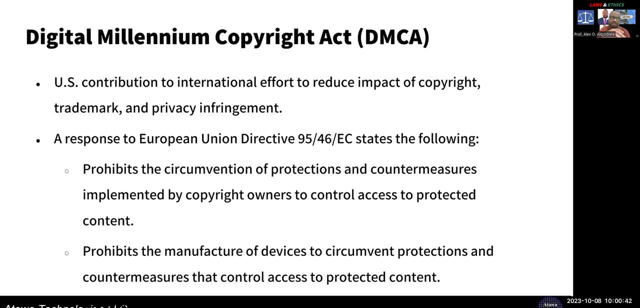 do you dispute intellectual property, and then it goes on. so now millennium copyright act, DMCA- this is from. this is a US law. it has to do with efforts to reduce the impact of copyright, trademark and privacy infringement right. so you had another European one. so they're trying to make sure they are compliant with it. 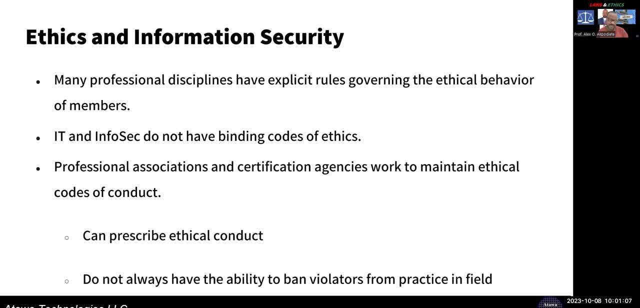 all right. so ethics and information security: um, there might not be any like binary codes for IT, but their own prescribed ethical conducts. In other words, you're going to be a member of our organization, You're going to be certified with us. This is what you must abide. 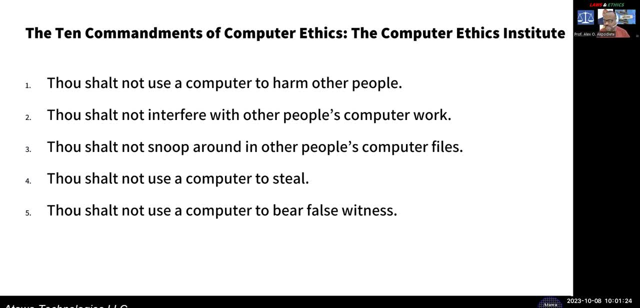 by. So this is called the Ten Commandments of Computer Ethics by the Computer Ethics Institute. There's ten, just like the Ten Commandments, the Biblical Ten Commandments or the Jewish one. also right, You should not use your computer to harm other people. 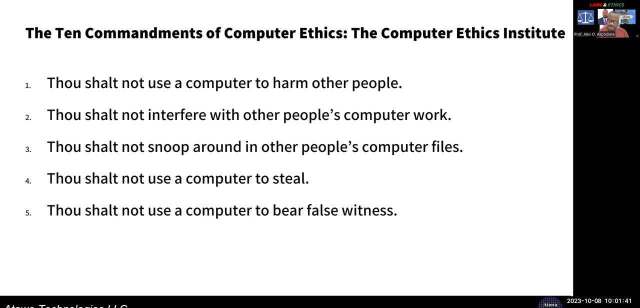 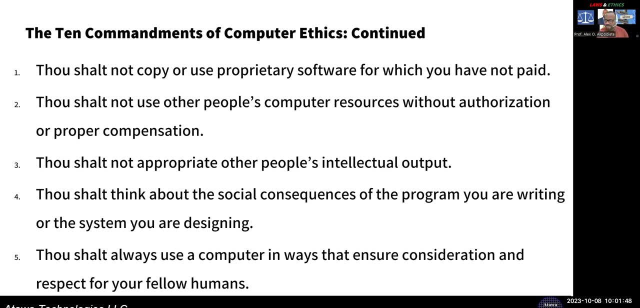 to interfere with other people's work. snoop other people's computers' files, steal files, be a false witness. copy proprietary software without paying for it. use other people's computer resources without authorization. do not appropriate somebody else's intellectual property. 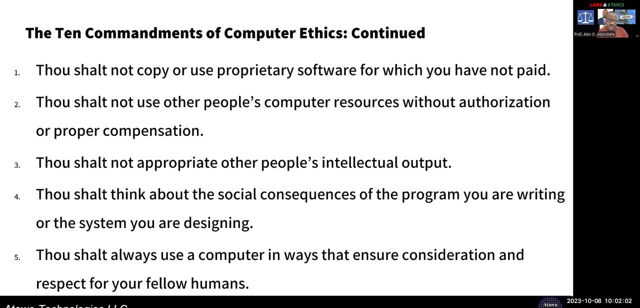 right. And then, of course, you should not think. thou shalt think about the social consequences of the program you're writing or the system you are designing. Thou shalt always use a computer in ways that ensure consideration and respect for your fellow humans. 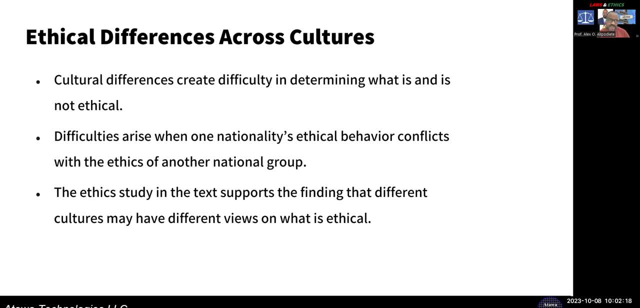 I'm also a member of the Humanistic Leadership Academy, HLA. So when I see that last portion I smile because myself and my fellow professors in the cohort, or even when I was doing my MBA, I had to be a member of the MBA. We understand. 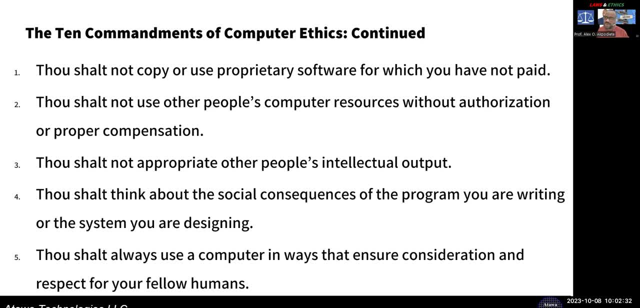 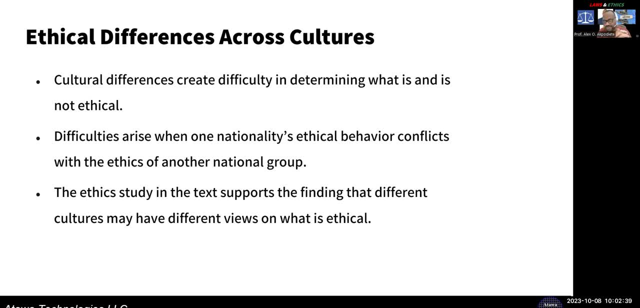 this part about things that consider your fellow human beings right- Making businesses work for everybody, All right. so the issue now is that different cultures have different ethics. So what exactly is and it's not ethical? If you see the little slide to your right of your screen. 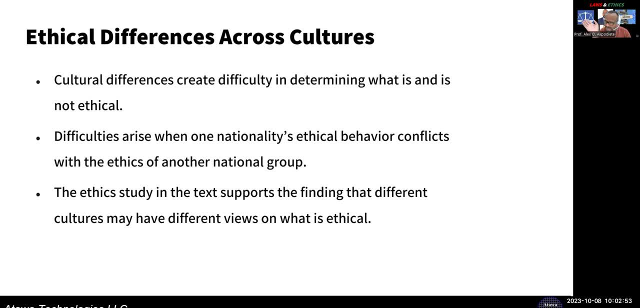 where you've got- I don't know how you're looking at. you've got the skills of justice and you've got a three-way arrow I have on there. One says right, wrong depends. Some countries, bribery is part of doing business. 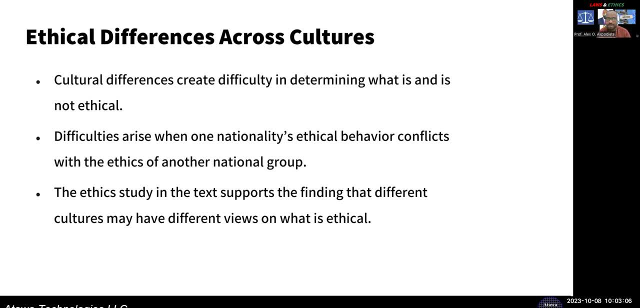 Some people say having more than one wife is allowed in a culture, or whatever. One girlfriend using software you didn't pay for. So in the study in ethics and as I said in 2001, I started teaching business law and ethics at the university in South. 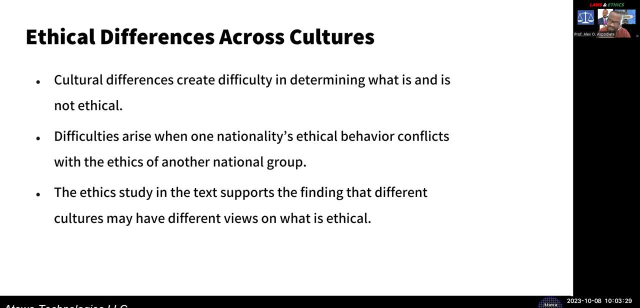 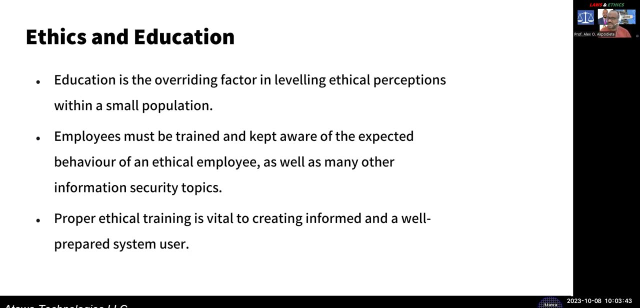 Florida To today. the whole idea is that different cultures may have different views on what is ethical. So just understand it, because ethics has a lot to do with cultural morals or morals right. So education is the overriding factor in leveling our perceptions of ethics within any 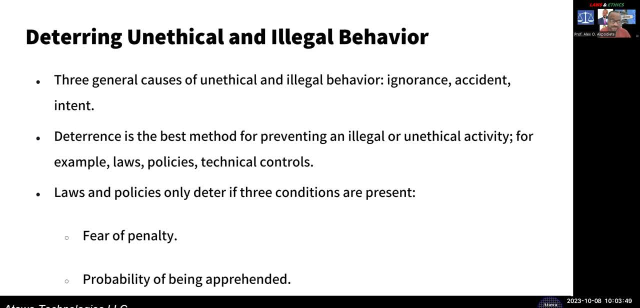 kind of population. So you must train your employees. It's very, very important. But to deter ethical and illegal behavior you first have to understand what causes people to behave in an unethical or an illegal manner. It's always said that people behave. 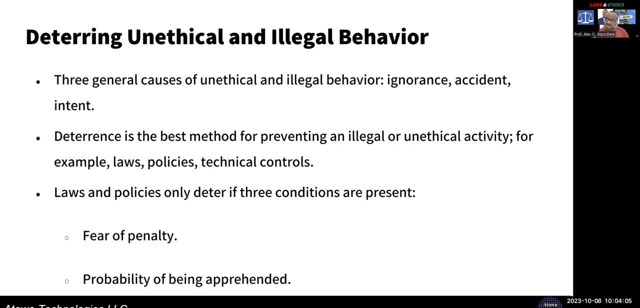 three things can make people behave: illegally: or unethical Ignorance, or by accident, or intent. So usually in law to commit a crime you have to have two things called the mens rea right, which is your mind and intent, and then the actus rea. 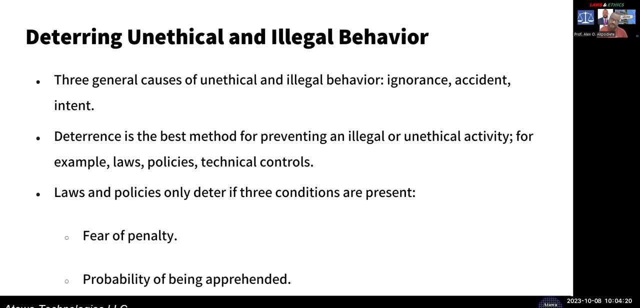 the actual act that you've done. right to be convicted, right. So so deterrence is the best method to prevent this from happening, right, whether it be by laws, policies or technical controls actually in an organization. So it 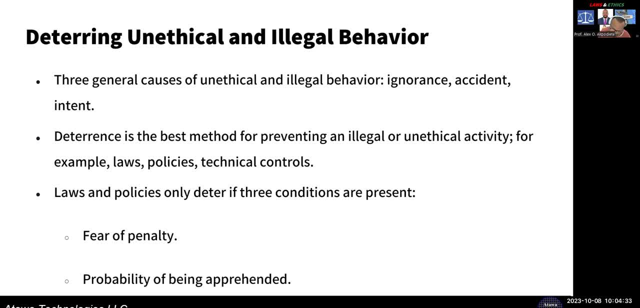 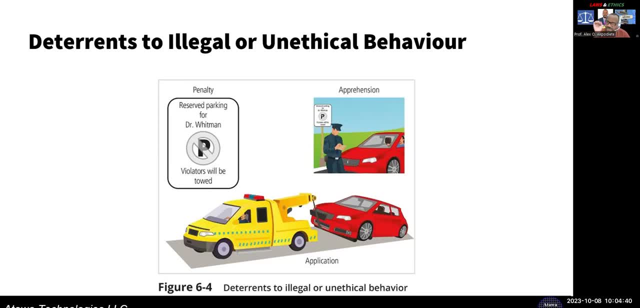 must be fair and you have fear of penalty, probability of being apprehended. Look at this chart in here: Speeding tickets. So, like in some parts of the world, even if you don't even see a police, you're going to get a ticket in your mail. in your mail or in. 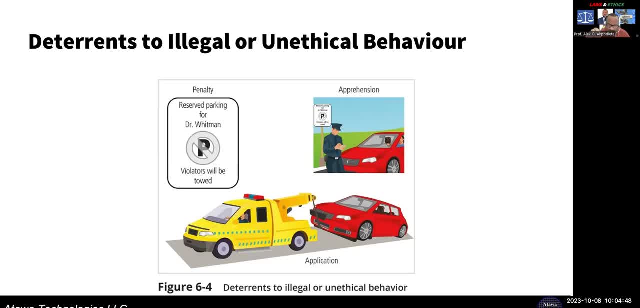 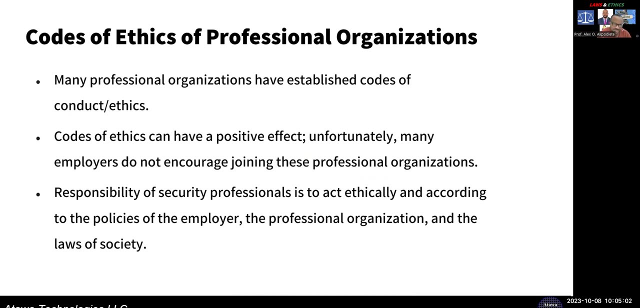 your box if you go past the speed limit with a camera. So if you know that you can be apprehended and you know that it's a penalty and you know that it's applied universally, you know these are deterrents to ethical or illegal behavior. So, as 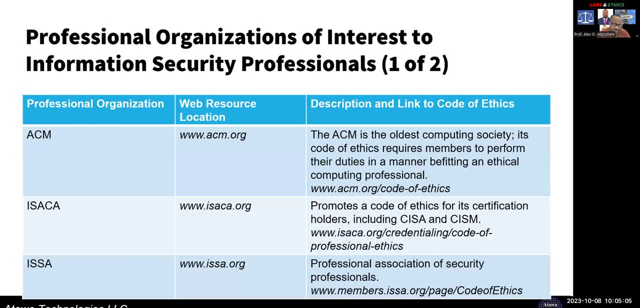 I said, most organizations have their own code of conduct or ethics. We've got the ACM, ISACA, which I belong to, ISS. I have the CISM certification from ISACA- Certified Information Security Manager. You have the ISC2 also. You have SANS. The SANS is pretty good. 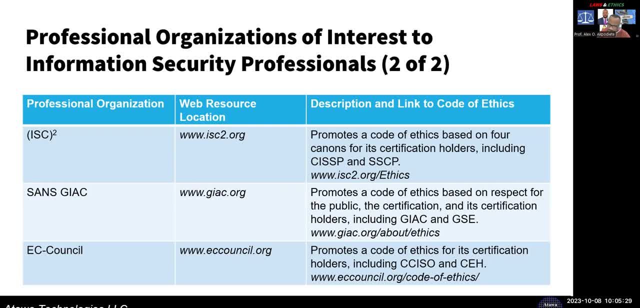 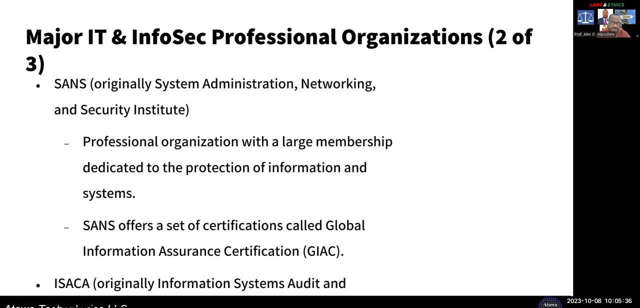 A lot of their certifications are expensive. You have the UC Council. They do the ethical hacking right, certification right. This is the ACM Computing Machinery. They have their own separate code of ethics. You have the SANS, So systems administration network. 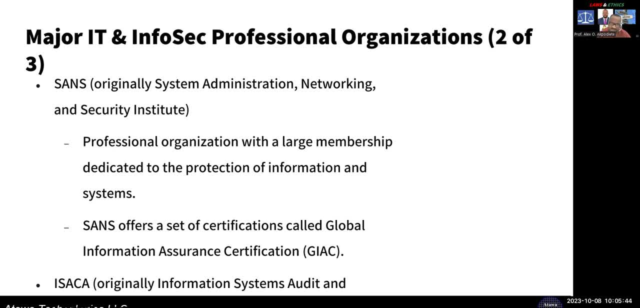 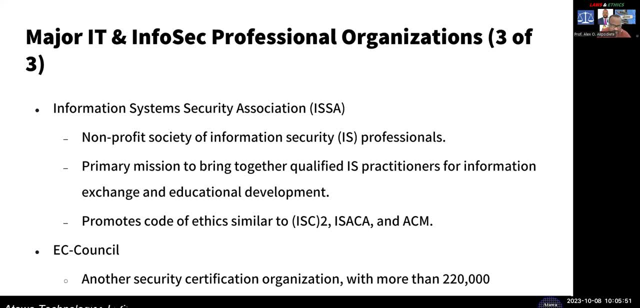 security. that was the original name for SANS And it's a very large organization, very reputable. The ISACA: as I said, I'm a member of this, but there are branches in UAE and in the US, And then the EC. 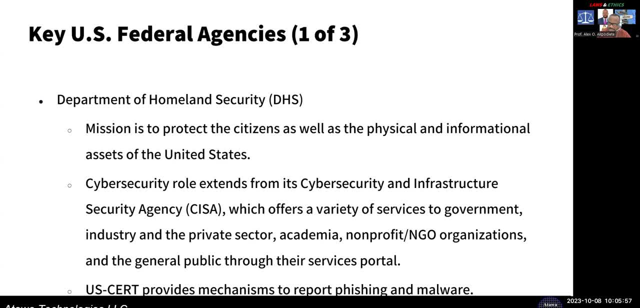 Council also. So Homeland Security I already talked about as related to Patriot Act, all kind of 9-11, right Protect American citizens as well as physical information assets of the United States. So cybersecurity rule extends From the cybersecurity infrastructure security agency.